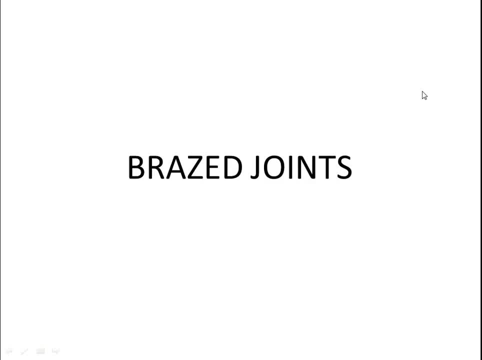 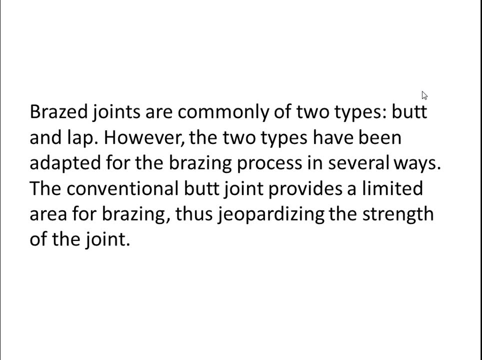 Let's talk about braze joints. Actually, braze joints are commonly of two types, and first one is bar joint and second one is lap joint. However, the two types have been adopted for brazing processes in several ways. The conventional bar joint provides a limited area for brazing. 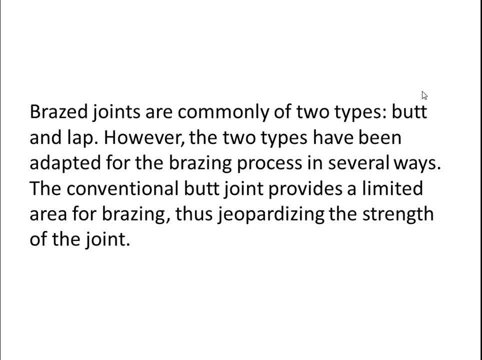 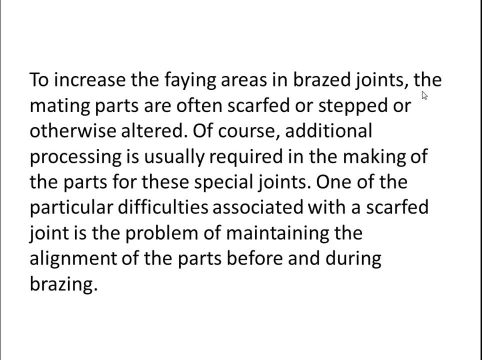 thus jeopardizing the strength of the part of the joint. To increase the faying areas in braze joints, the mating parts are often scarped or stepped or otherwise altered. Of course, additional processing is usually required in the making of the parts for these special joints. One: 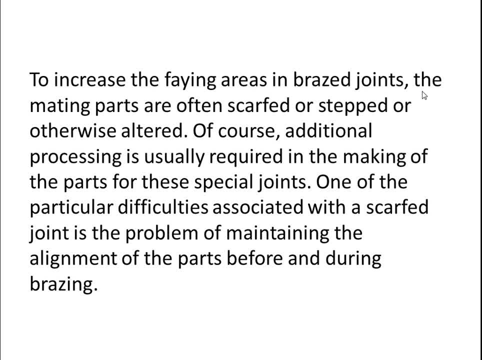 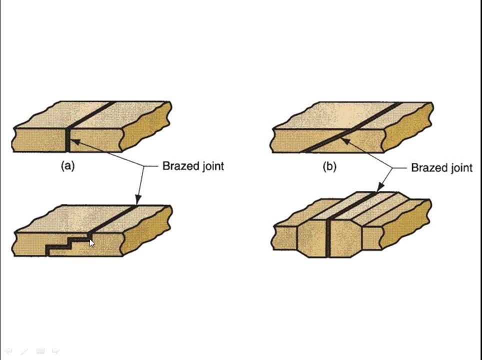 of the particular difficulties associated with a special joint is that it is difficult to make a scarred joint. It is a problem of maintaining the alignment of the parts before and during brazing, And there are figures about joint. So this is joint, another joint and this one is one. 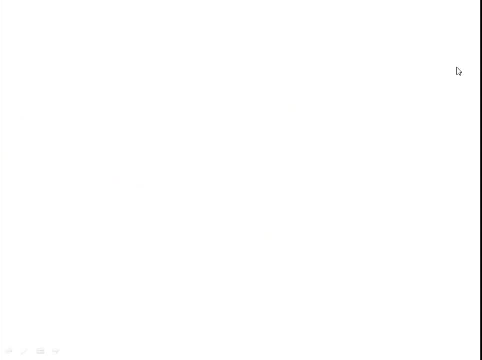 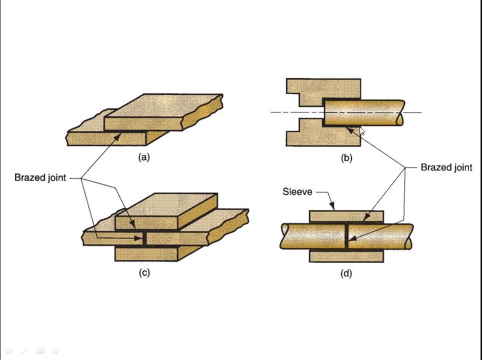 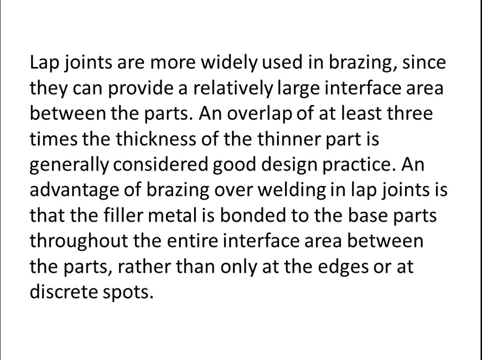 type of joint and this is another joint, And there are lap joints and some other examples of lap joints. Lap joints are more widely used in brazing since they can provide a relatively large interface area between the parts, An overlap of at least three times the thickness of the thinner. 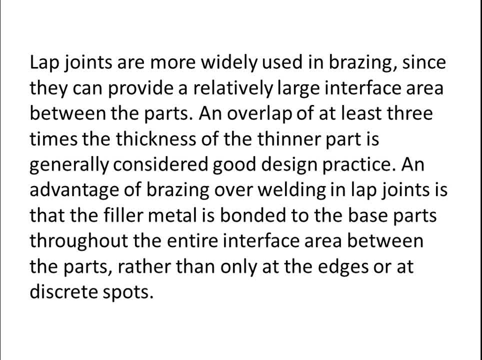 part is generally considered good design practice. An advantage of brazing over welding in lap joints is that the filler may be filled in to the inner side of the brazed joints and therefore the thinness may not be fully filled in to the inner side of the brazed joints And the brazing of this 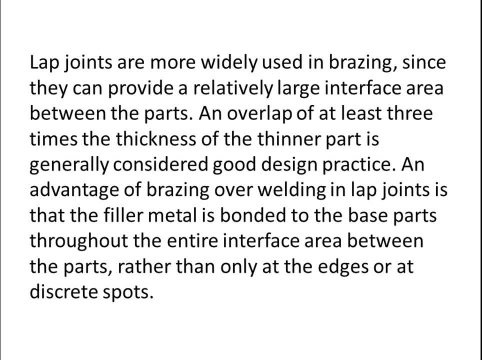 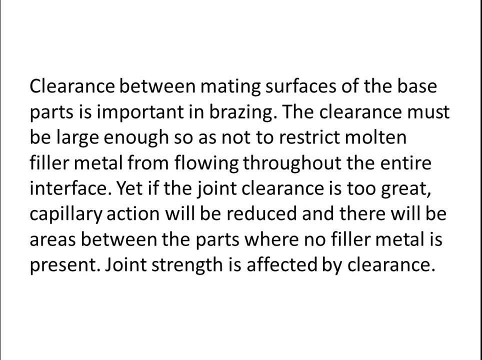 metal is bonded to the base parts throughout the entire interface area between the parts, rather than only at the edges or at discrete spots. Clearance between meeting surfaces of the base parts is important in brazing. The clearance must be large enough so as not to restrict molten filler metal from flowing.